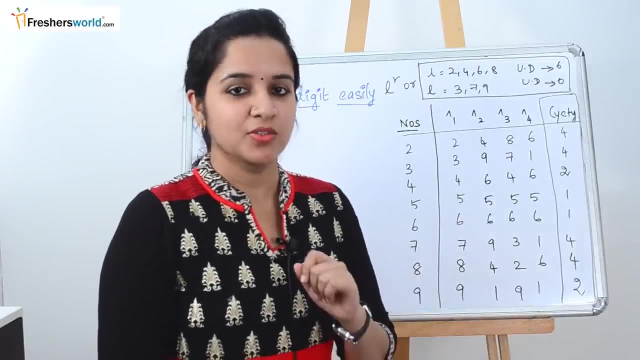 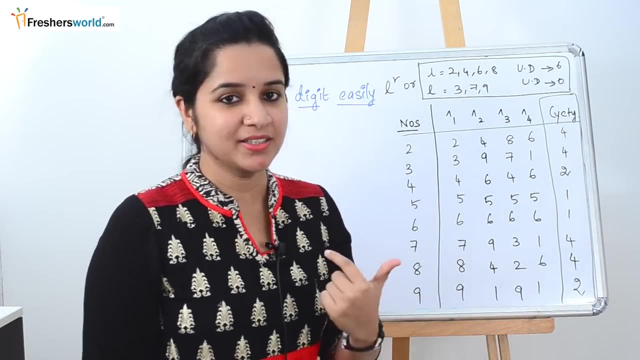 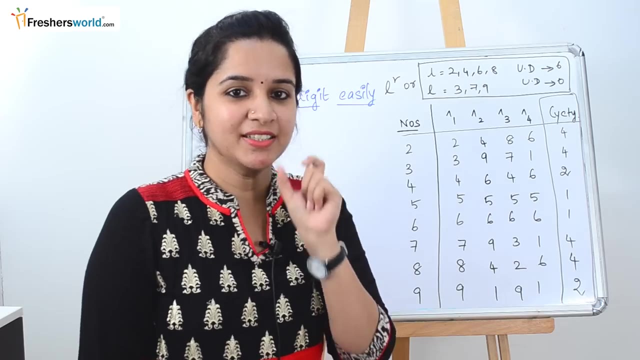 So first thing is the cyclicity of the numbers. So what is the cyclicity of the numbers is nothing but 2 power 1, 2 power 2, 2 power 3, 2 power 4.. You can see that there is a pattern in this. After 2 power 4 is nothing but 2 power 5, which is nothing but 32.. So again, the units digit end in 2.. So again, if you see 2 power 6, the units digit end in 4.. So the 2, 4, 8, 6 pattern repeat every 4 times. So the cyclicity of 2 is nothing but 4.. 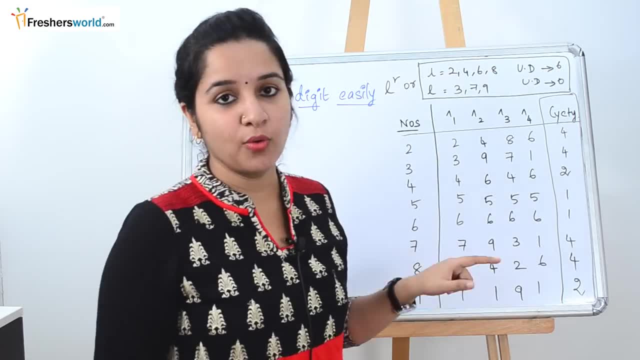 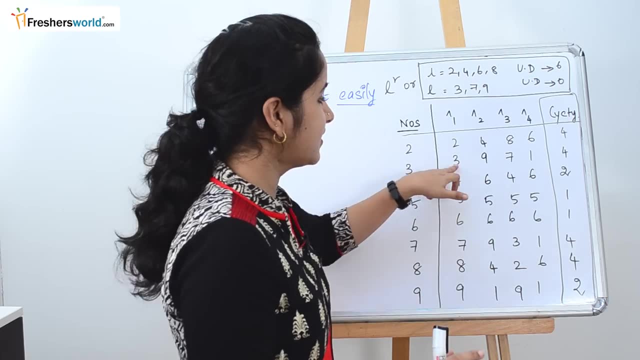 So in case of 3, you can see after 3 power 4, in 3 power 5, again we get the units digit as 3.. So after every 4 times you can see that 3971 in the units digit will be again replaced. 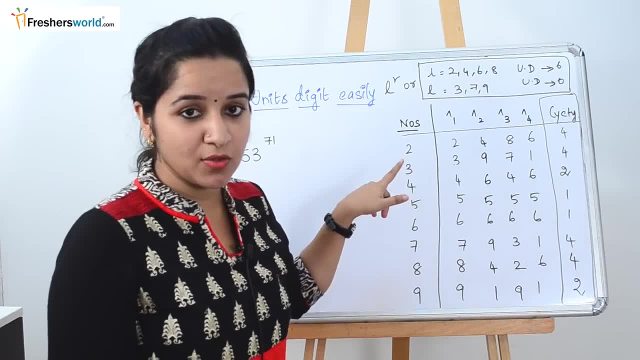 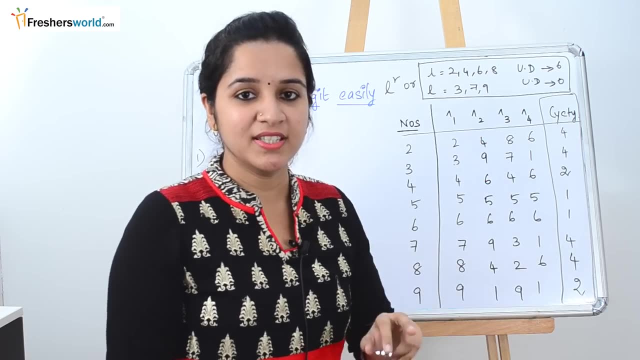 So hence the cyclicity, for it is 4.. Similarly, in case of 4, we know that 4 power 1 is 4, 4 power 2 is nothing but 16,, 4 power 3 is nothing but 4,, 4 is 16, 16, 4 is 64.. 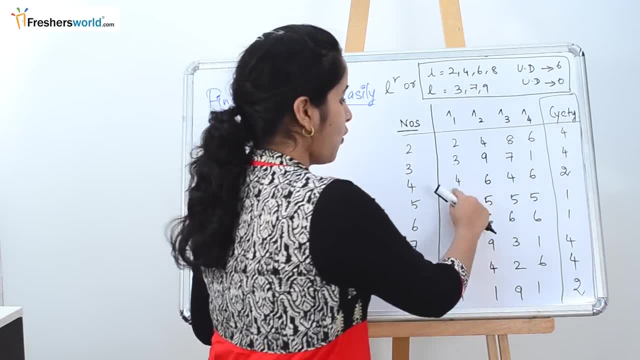 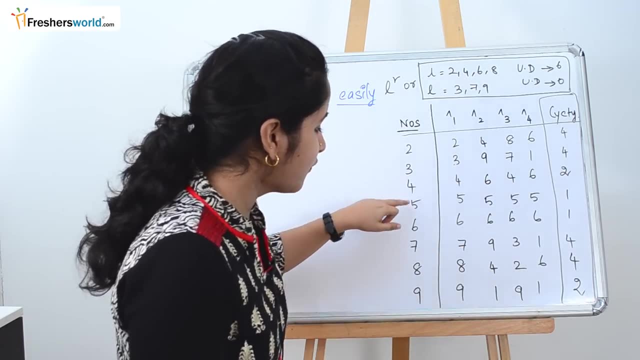 Again, if you see the units digit is 4.. So 4, 6, 4, 6 will be done after every 2 times, So the cyclicity is nothing but 2.. But in case of 5 and 6, whatever be the powers, you can see that the same digit is repeated. So the cyclicity is nothing but 1, 1 in both case of 5 and 6.. In case of 7, you can see the cycle is 4.. In case of 8, you know it is 4.. And for 9,, 9 and 1 will be repeated. 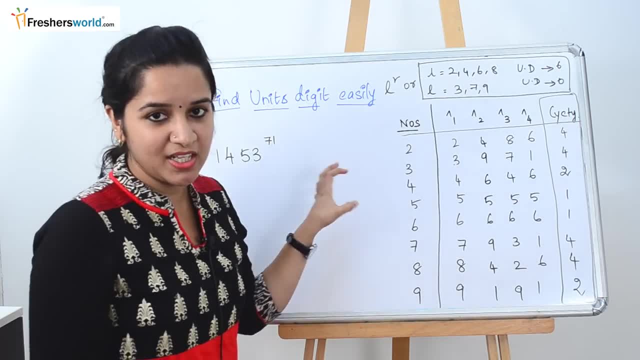 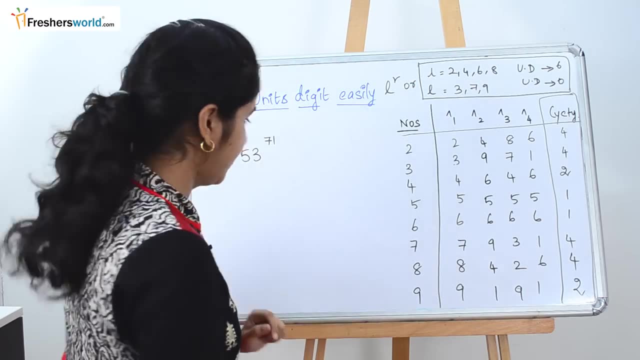 So you should know this table to solve the sums very easily here. So there is also another concept here, So which I will be explaining while solving the sum. So let's get started. So the question that they have given is: find the units digit of 1453 to the power 71.. 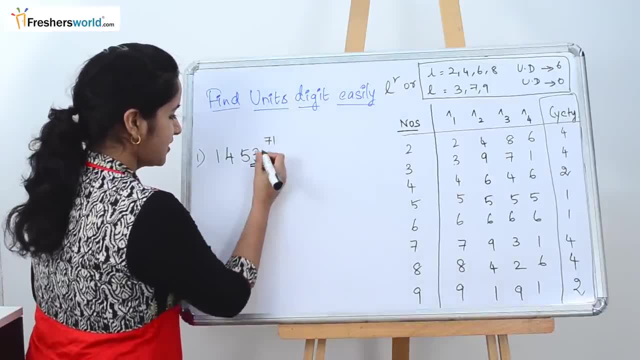 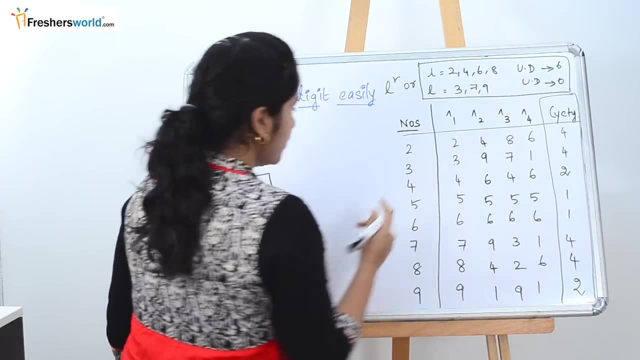 So the first step is that take this digit. So this is nothing, but the last digit is 3.. So the cyclicity of 3 is nothing but 4.. So 4 times in case of 3 is repeated. 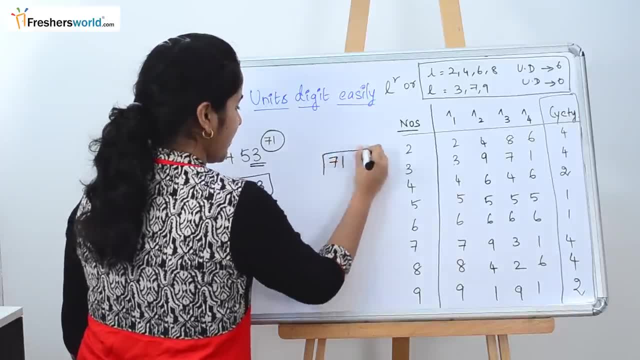 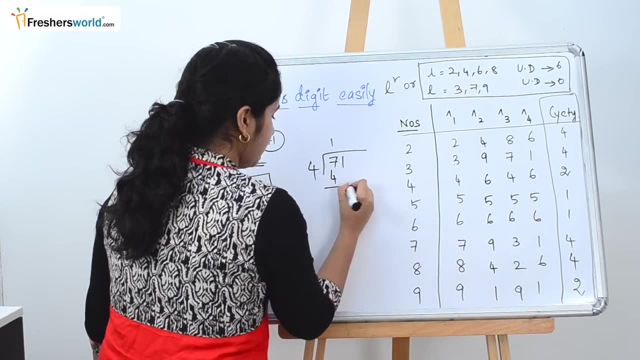 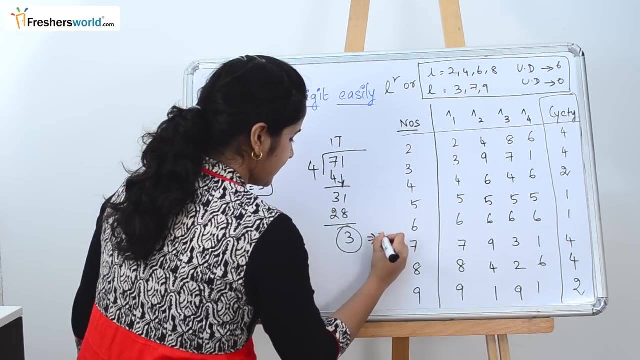 So now you have to take the power, Divide 71 by 4.. What is this 4?? This is nothing but the cyclicity of 3.. So 4, 1's are 4, 31, 7's are 28.. So the remainder is 3.. 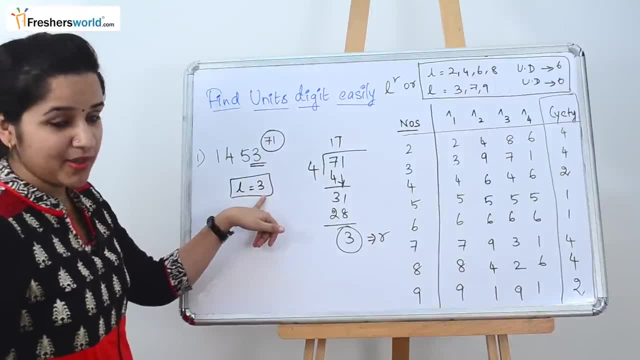 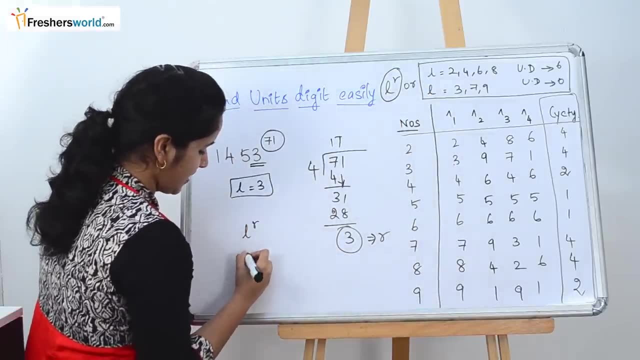 So once you get the l, as, you have a value as 3 and remainder you have a value as 3.. So we are going to use this formula: l power r, which is nothing but 3 power 3.. We know 3, 3's are 9, 9: 3's are 27.. 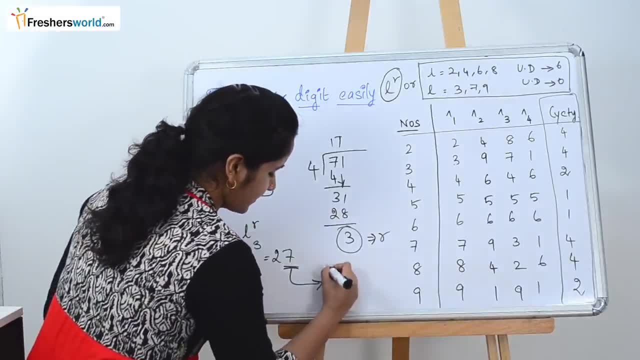 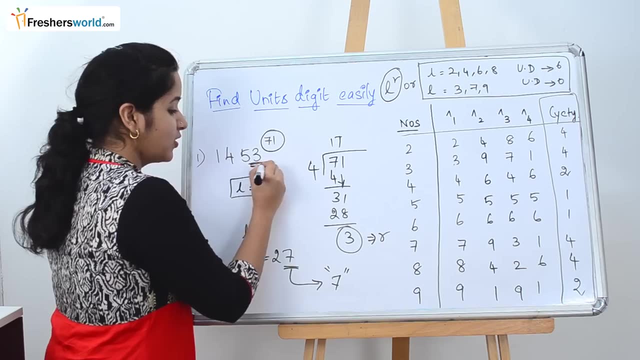 So the units digit is nothing but 3.. So this is nothing but 7.. So what did we do here? First we have to find l and r. So l is nothing but the last digit of the given number. 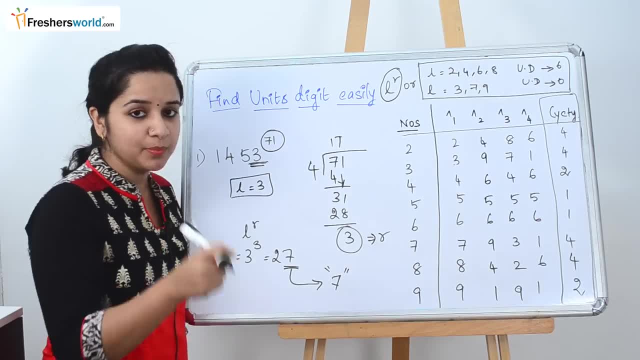 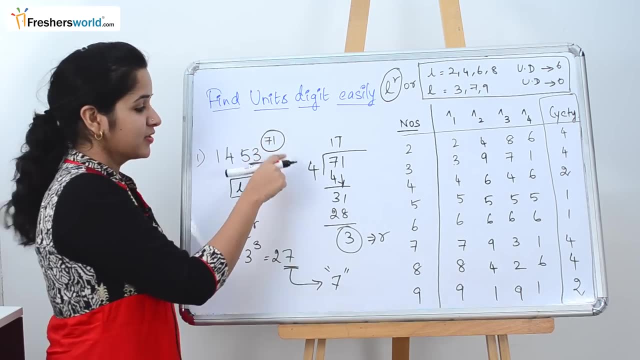 So you write it as l is equal to 3.. Then you should know the cyclicity of that particular number, Which is nothing, but for 3, it is 4.. So use that number to divide the power. So 71 divided by 4, the remainder is 3.. 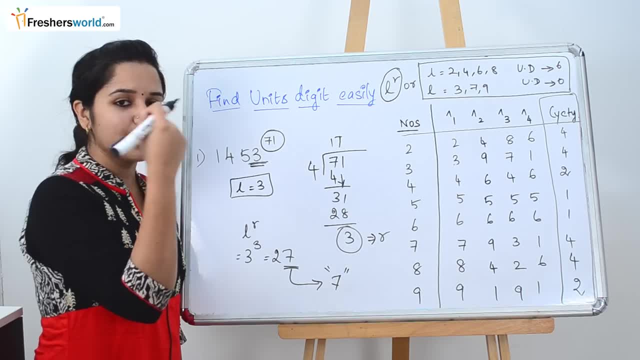 So you know l, you know r, So l power r is nothing but 3 power 3, which is 27.. So units digit is nothing but 3 power 3, which is 27.. So they are asking for the units digit. 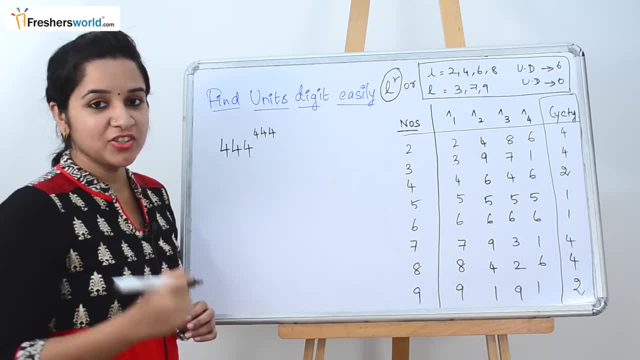 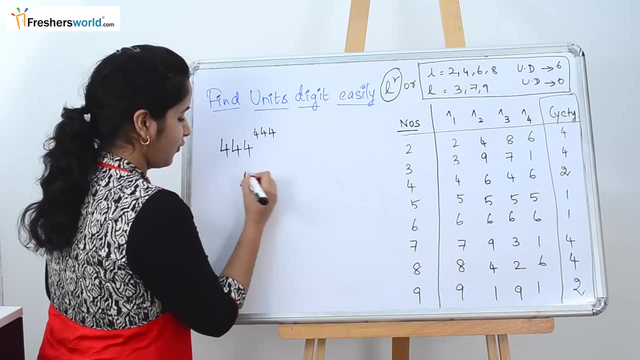 So units digit is nothing but 7.. Let's solve another problem. So the question that they have given is 444 to the power 444, find the units digit of it. So what is the first step? l is equal to 4.. 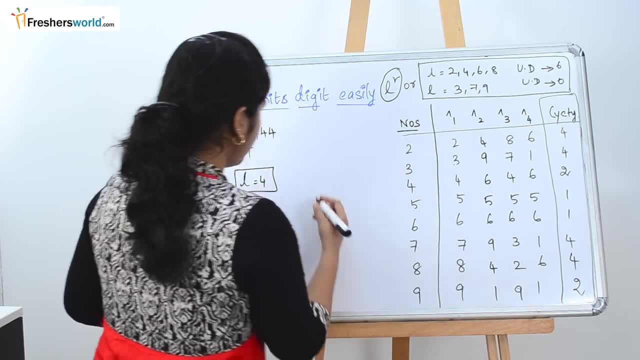 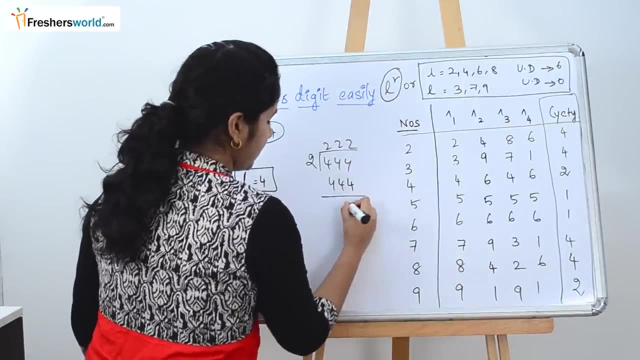 So next, for 4, the cyclicity is nothing but 2.. So you are going to divide the power by 2.. 2- 444.. So the remainder is 0.. So what do we do in the case when the remainder is 0?? 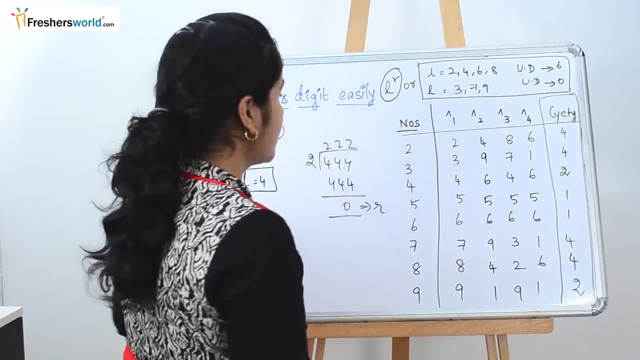 So what do we do in the case when the remainder is 0?? Then comes these two steps: If your remainder is 0, and if your l value comes between 2,, 4,, 6,, 8, and if your l value comes between 2,, 4,, 6,, 8,. 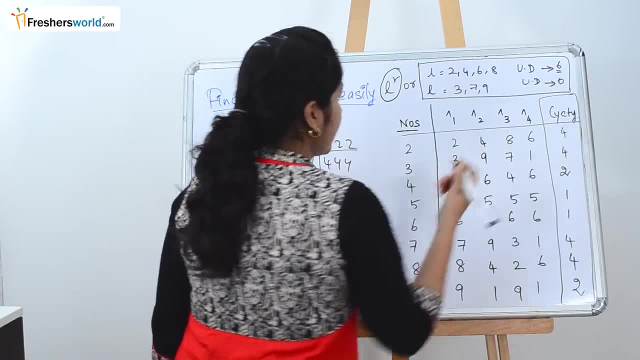 then your units digit will always end in 6.. then your units digit will always end in 6.. If your last digit is 3,, 7 or 9, then your units digit is 0.. then your units digit is 0.. 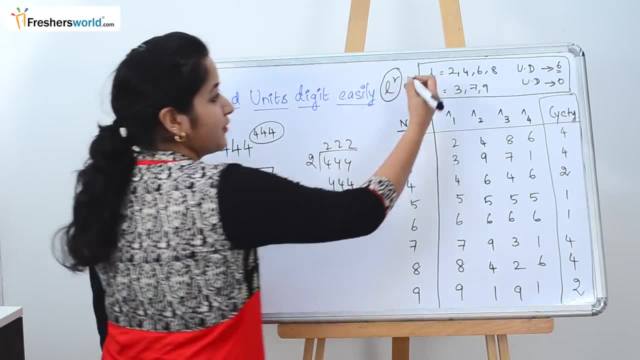 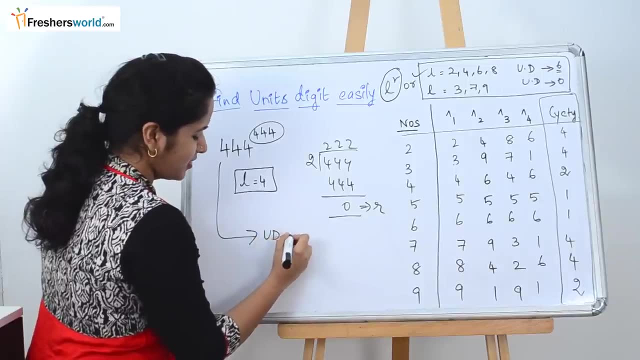 So here the l value is nothing but 4.. So it comes into the first category. So l is equal to 4, then the units digit is 6.. So directly you can write that units digit is 6 instead of solving anything. 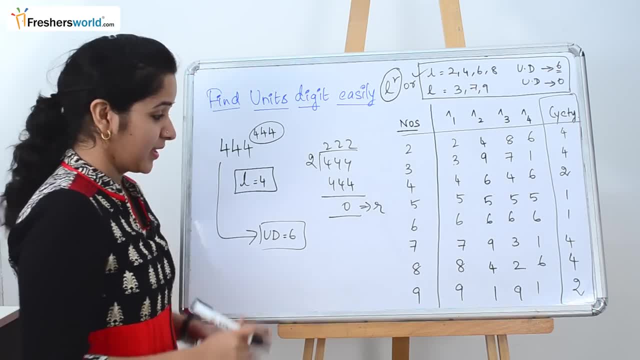 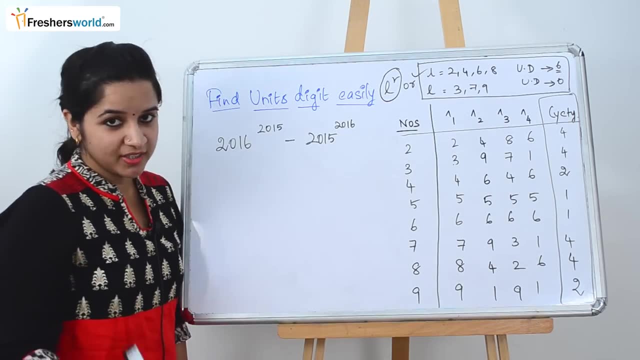 that units digit is 6 instead of solving anything. So this is a very simple way of solving the sum. This applies only when your remainder is 0.. This applies only when your remainder is 0.. Let's solve another problem. The question that they have given is: 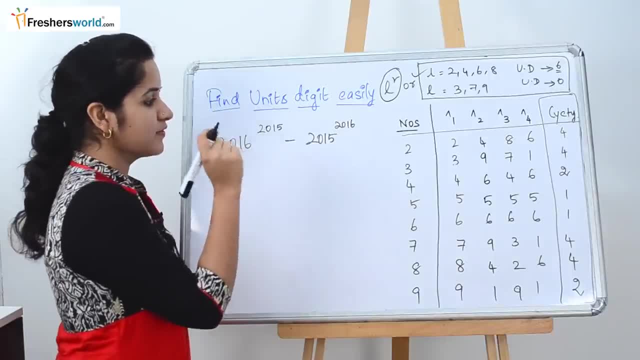 2016 to the power 2015. minus 2015 to the power 2016.. minus 2015 to the power 2016.. We have to find the units digit of the whole sum. So let's get started with this. 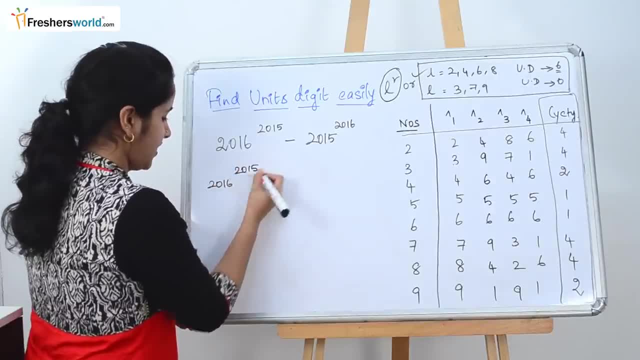 So 2016 to the power, 2015.. So last digit is 6.. So last digit is 6.. For 6,, the cyclicity is 1. So we have to divide it by 2015,. 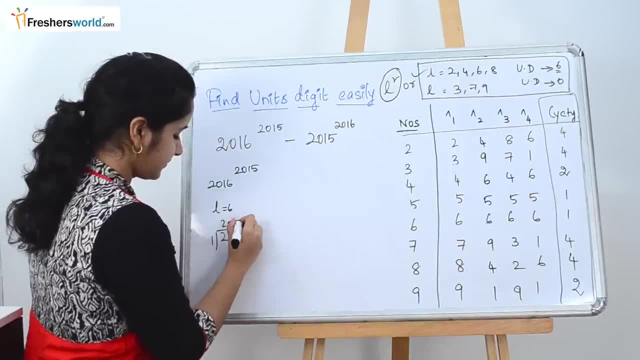 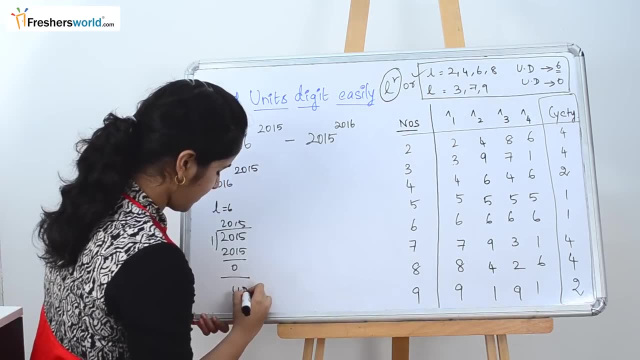 So we have to divide it by 2015,, which is nothing, but your remainder is going to be 0.. So, as l is equal to 6, the units digit is nothing but 6.. the units digit is nothing but 6.. 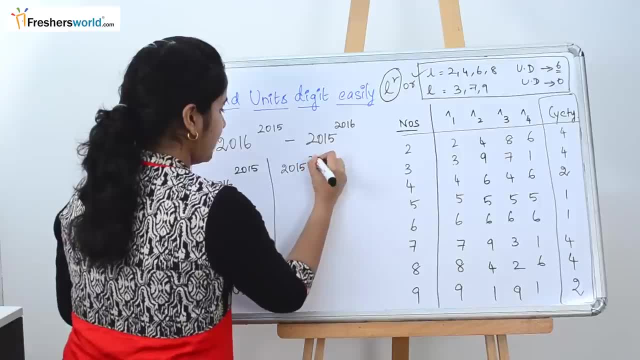 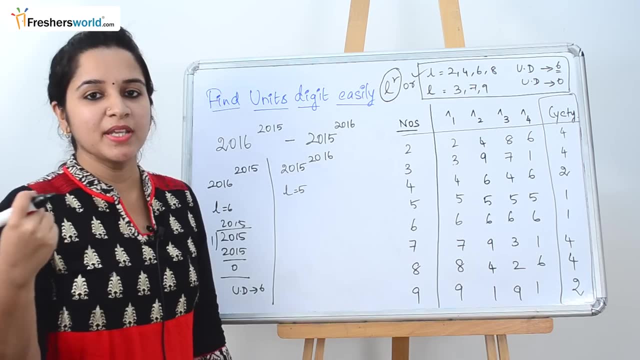 For this, 2015 to the power, 2016.. So l is equal to 5.. So, in case of 5, irrespective of whatever be your reminder is, or any case, your answer is always going to be 5.. That means: 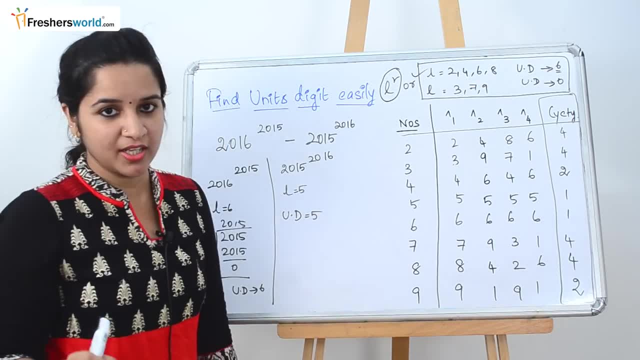 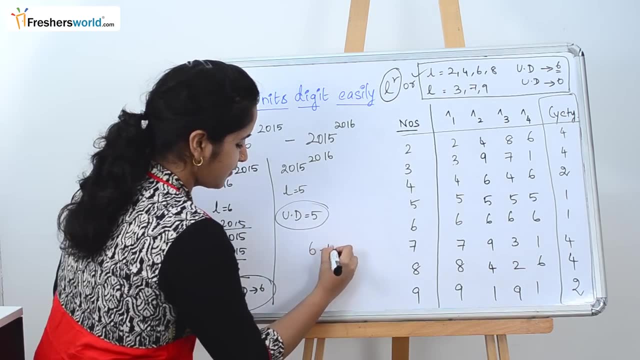 the units digit is always going to be 5.. This is the exception case only for the number 5.. So you know, the units digit here is 6 and here is 5.. So 6 minus 5 is equal to 1.. 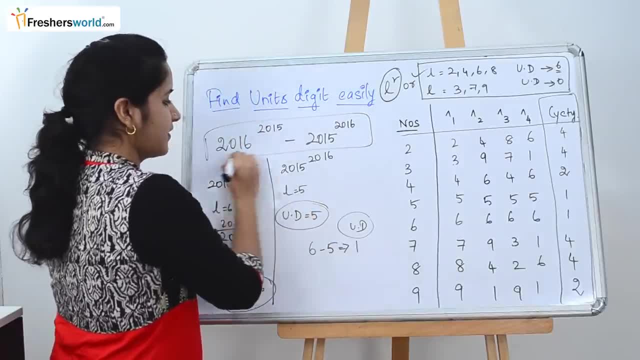 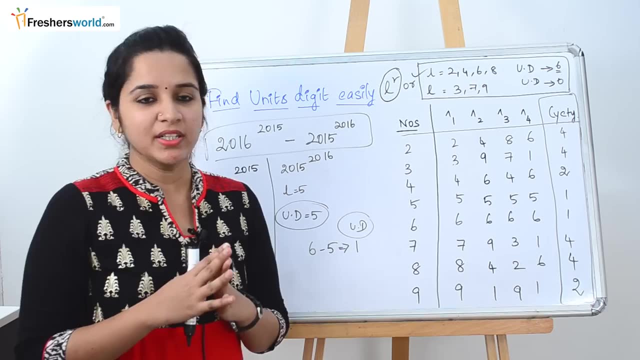 So the units digit for the overall sum that they have given here is nothing but 1.. In today's video, we dealt with how we can find the units digit very easily. In order to solve it, what you have to do is that.